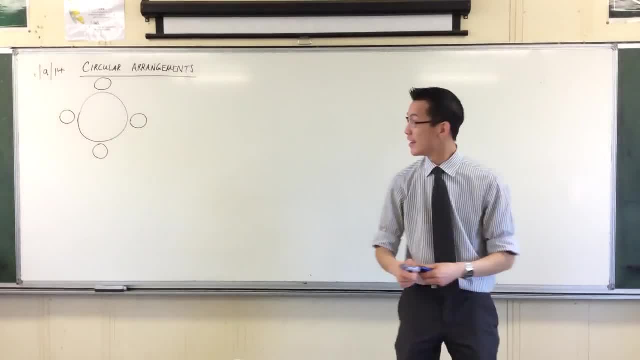 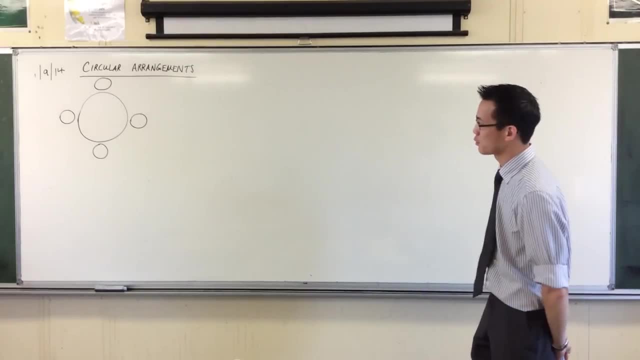 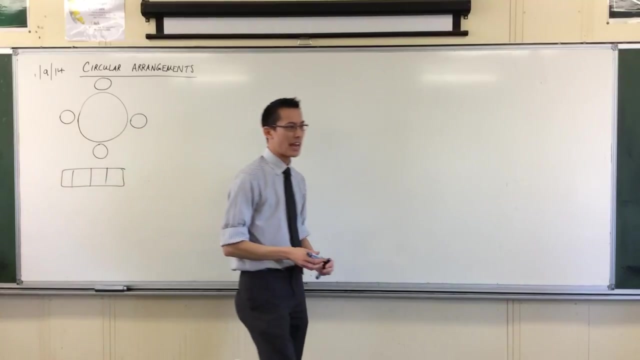 Here are the situations we're going to have a look at today. okay, Now just to review. before we get on to circles and, invariably, people sitting around tables, let's think about how we normally do arrangements. So we're thinking of things like this, okay, And you think of, you know, arranging. 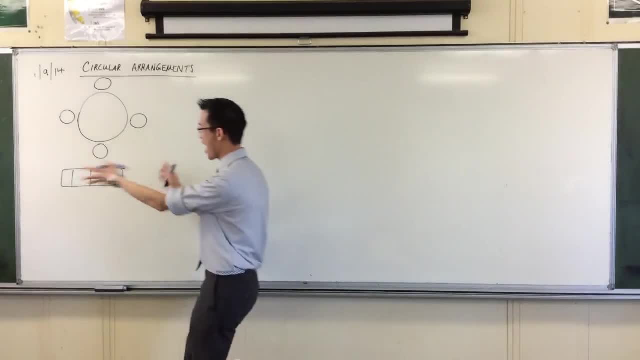 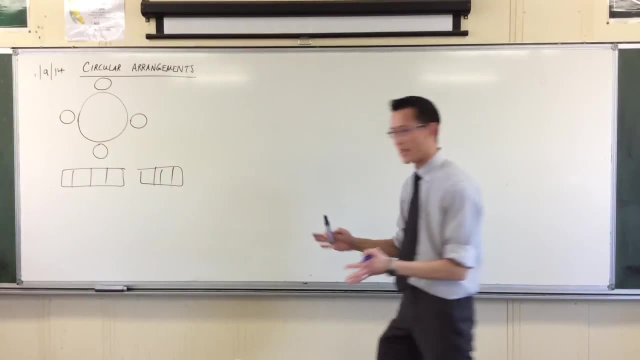 letters in a word, or arranging people in a line or putting people into teams, or you get the idea. okay. So thinking about something like, let's say something like this: okay, We're thinking of arrangements, we're thinking about not just combinations but wanting to know. okay, you know. 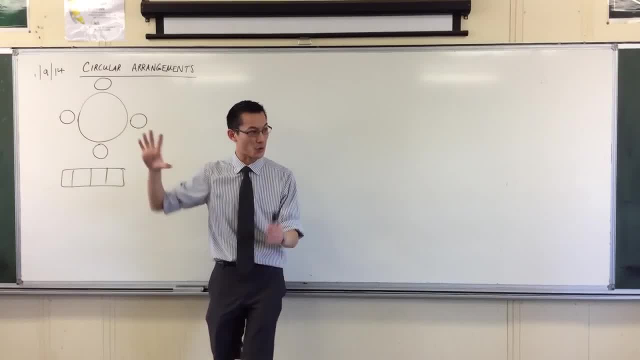 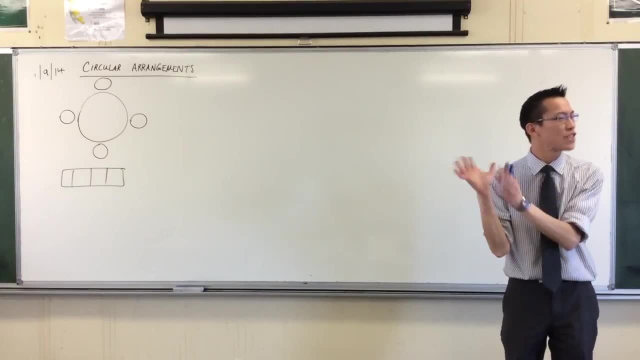 two people sitting in relation to each other in different orders. those matter okay, As anyone who has sat around a formal table will attest to. So this is permutations land, okay, When you see this, this is about permutations, So get your head back. 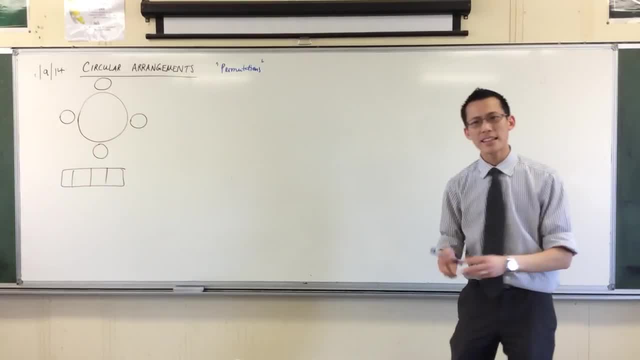 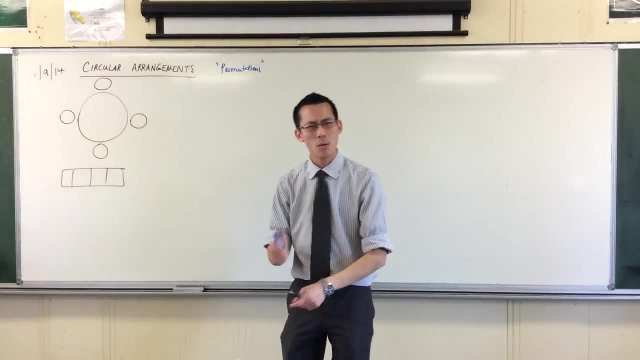 into that space right Now. let's think about just normal permutations in a line, right, If you've got four objects and you want to put them into four places, okay, What was the way that we worked out? There were no replacement, like we're actually putting real objects that can't be repeated. 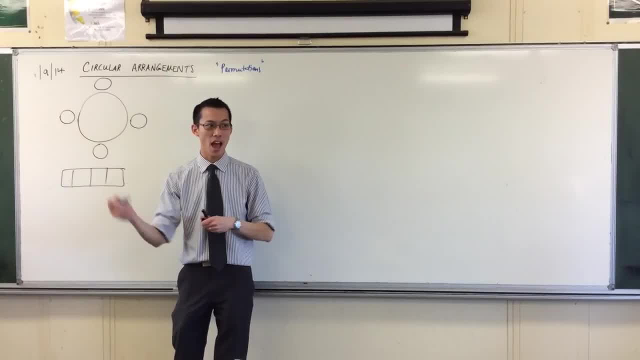 How many ways are there to pick something for the first spot? Answer: four ways, because you got four things right And then you got three more people left to put into the next spot, and then two and then one right. So this is where we got our factorial. 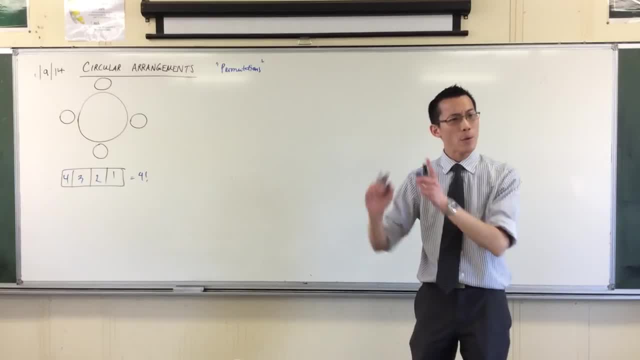 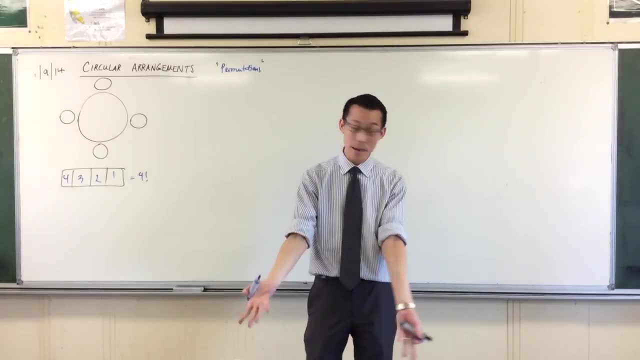 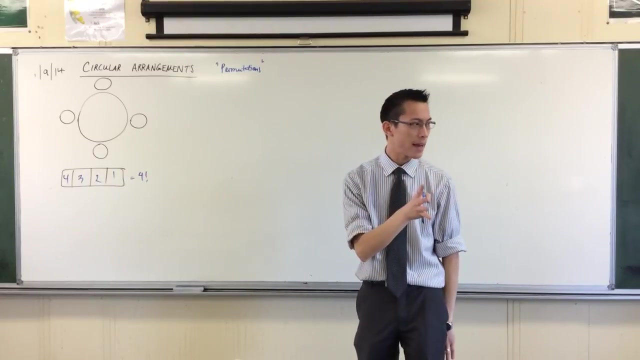 sort of notation from: okay, Now, when you have a look at a situation like this, okay, It looks so similar, You've still got four things, four people, and you've still got four places to put them into. okay, But there's a problem, there's a problem. We'll think about it like this: Let's, let's proceed. 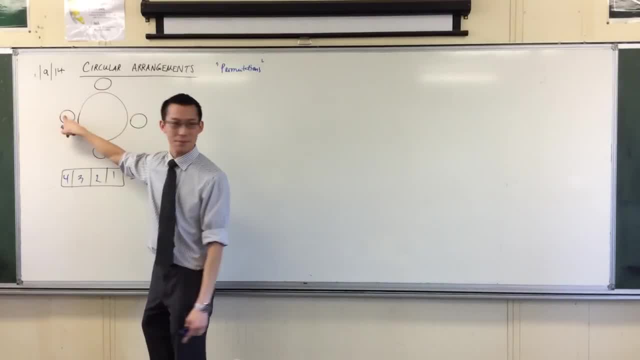 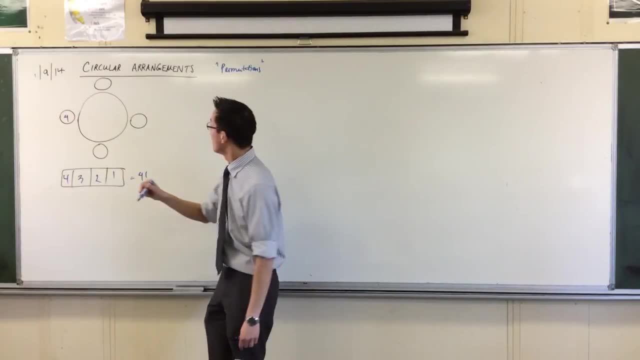 the way we did before. Pick a chair, any chair, like say this one: How many people can we put into this chair? There are four people I can put into this chair, right, And then you've got four people, And then you keep going around just like you went this way. You're like: well, I can put. 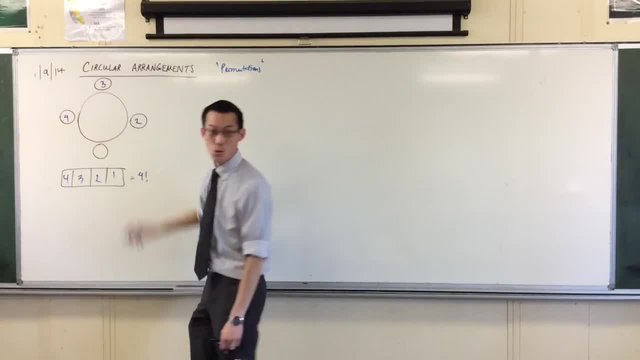 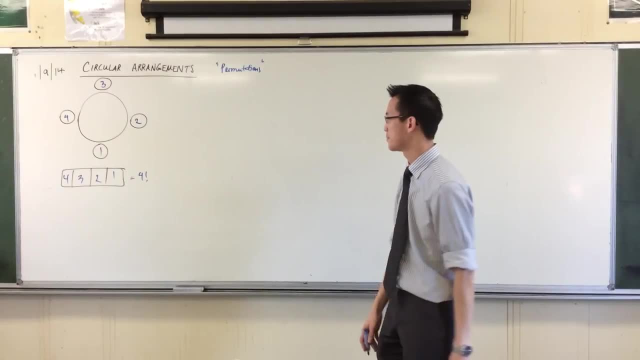 three more people into that chair, and then I've got two left And then whoever's last through the table gets to sit in that spot, right? So on the face of it, it looks like it's the same, okay, Except the problem is right. We, we care about order here. We care about order here, okay, And 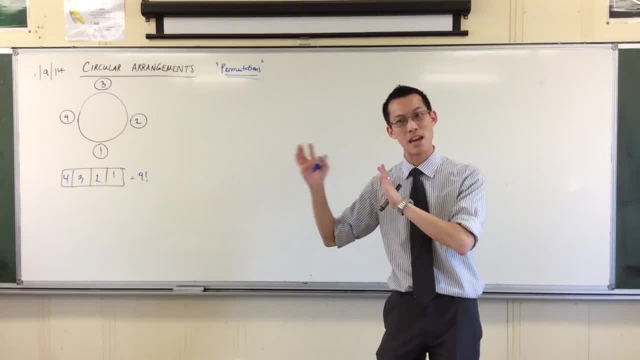 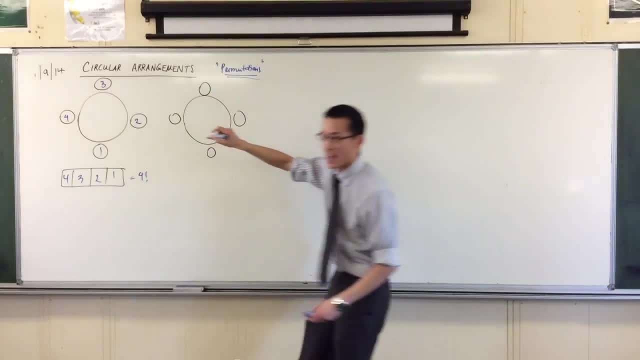 so, for example, if your four people have, you know, really imaginative names, like say: oh, I don't know- Savindha, Junga, Ellian and Martin- okay right, I just had to look and make sure. 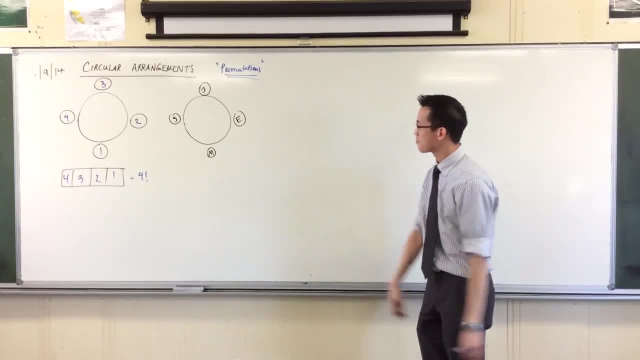 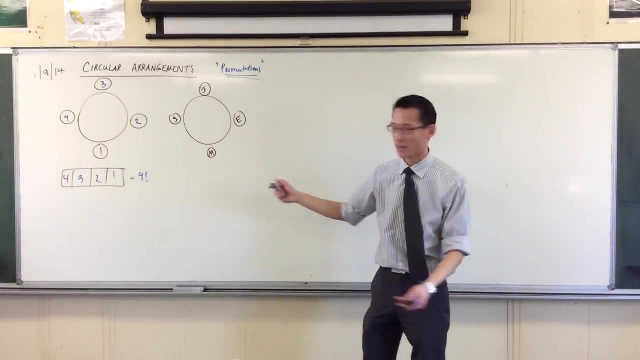 you all started with different letters. okay, There's one arrangement. right, There was my um, you know, first spot. Savindha got in first, then Junga was put in the second and Martin was the last to the table. Okay, But if, for instance, 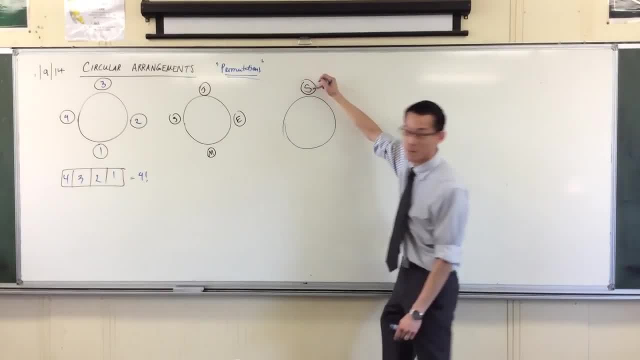 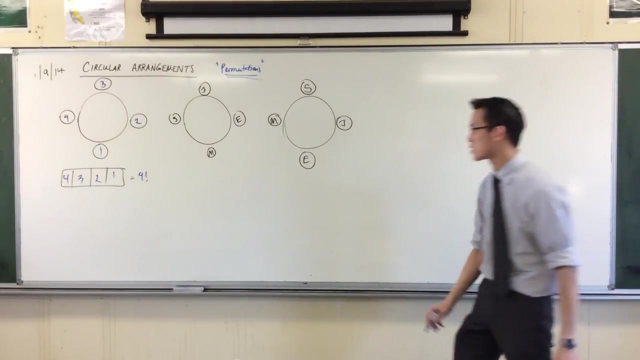 was first, but he decided actually he likes this table up- sorry, this chair up here right. And then Jünger still wanted to sit next to Svinda and he still wanted to sit here, and then Martin was still left over here. These arrangements are the same, right. 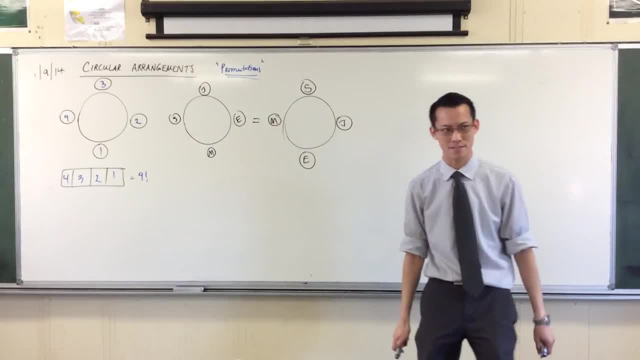 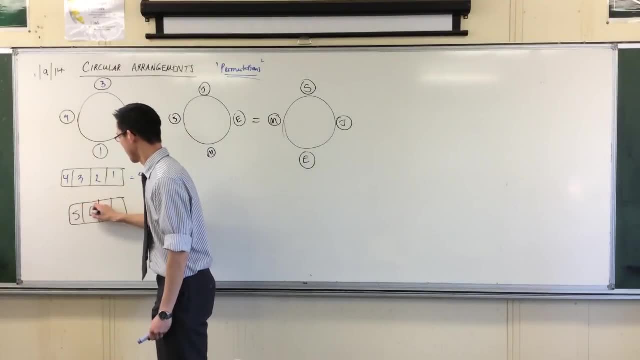 They're still the same arrangements. I'm just looking at it from a different angle, right? Just like you know, if I showed you this, okay, and so you look from this angle or look from that angle, it's like, well, the only difference between these two things is: 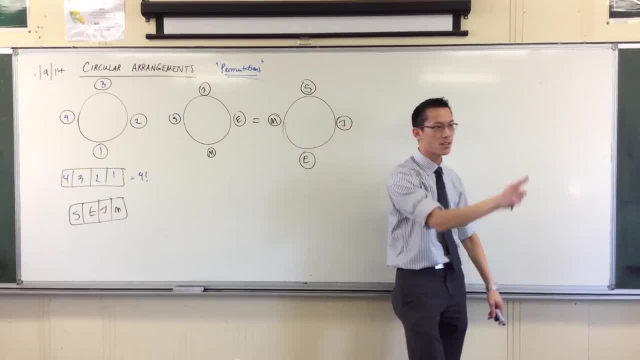 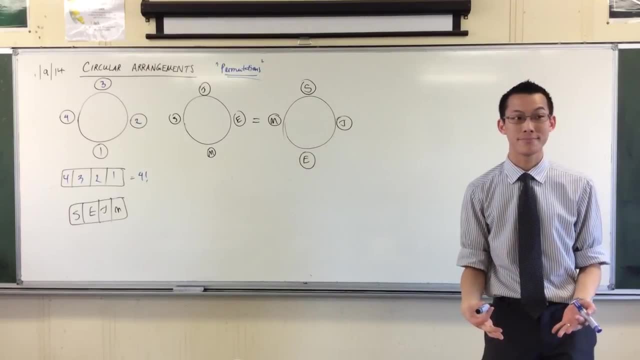 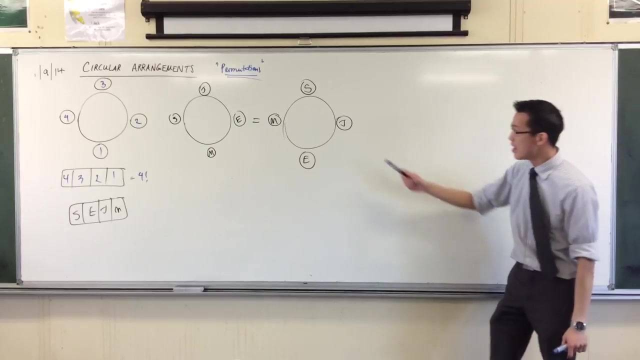 which side you're standing on. All I had to do was rotate. okay. Now here's the question: How many of these am I going to have? How many extras have I come up with? The answer is: I'll have four times as many as I should. I'll have three extras, right, Because I can. 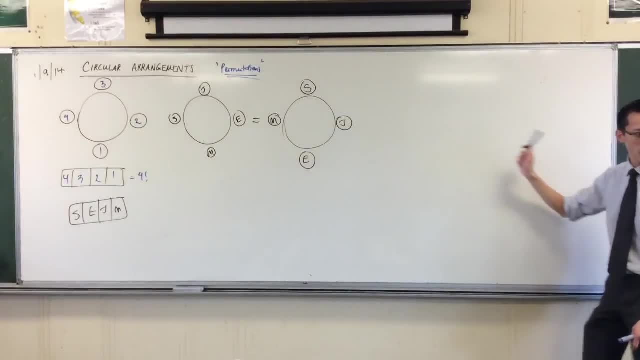 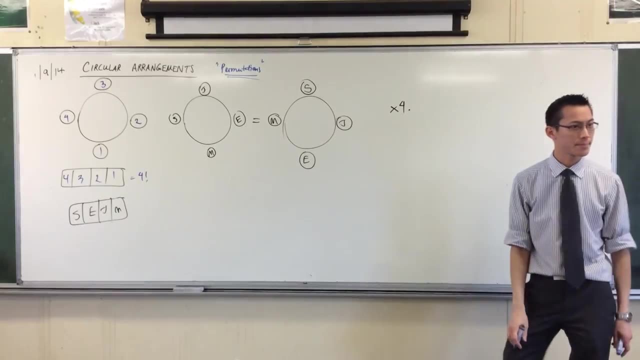 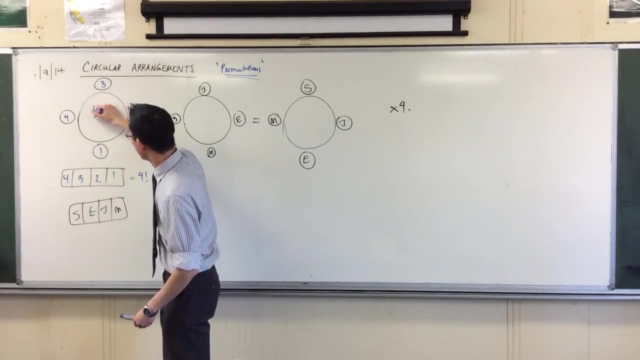 rotate this once and then twice and then three times. When I rotate the fourth time, I'll literally be back to here. okay, So I have four times too many, okay? So instead of four factorial, what I really have is four factorial on four right, And that four comes. 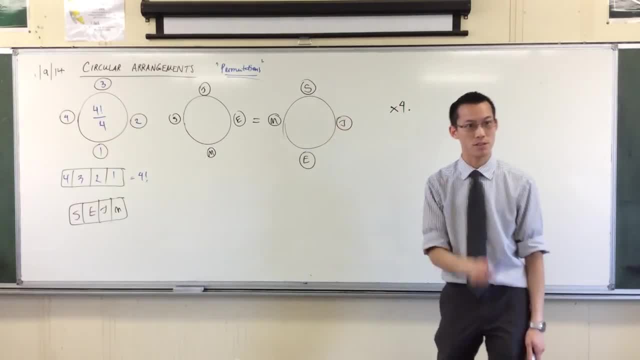 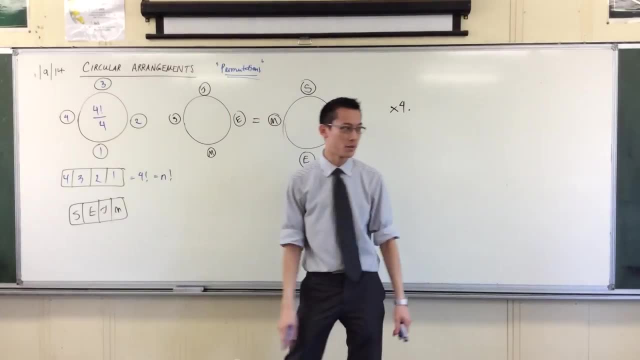 from the fact that I've got four spots and four people to put in those spots, okay. So, in fact, for an arrangement like this, rather than n factorial, I'm going to have four factorial, right, if you want to generalise, even though I don't see that much point in. 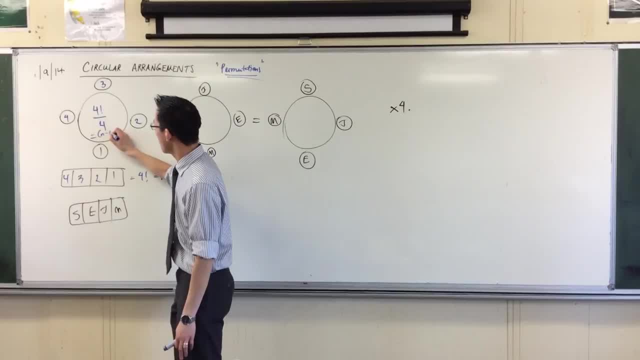 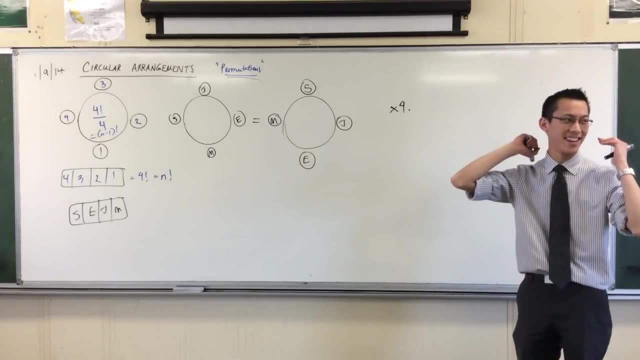 doing it. The general thing for this is: well, this is n minus one. factorial Simple. If you had twelve people to sit around an Asian banquet table, then there would be twelve minus one. eleven factorial ways to arrange them Make sense. Okay, now one more way. 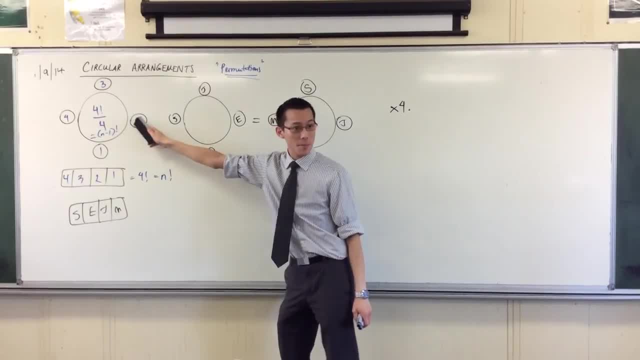 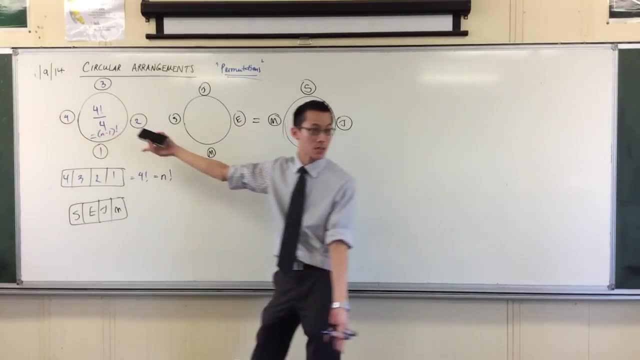 to think about it. okay, You can think about it in these terms- that you're doing this kind of set up, but then you're over-counting, right? So you correct by dividing by the number of people dividing, and that's what you end up with, The alternative, which is: 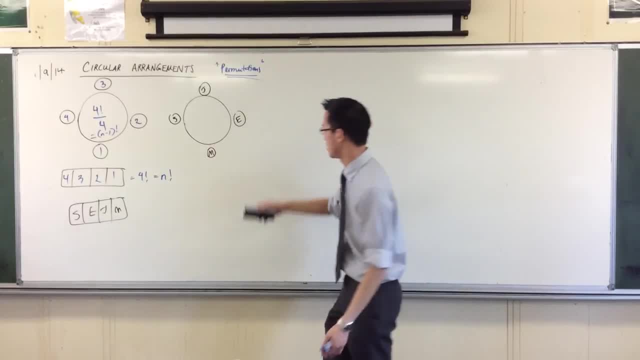 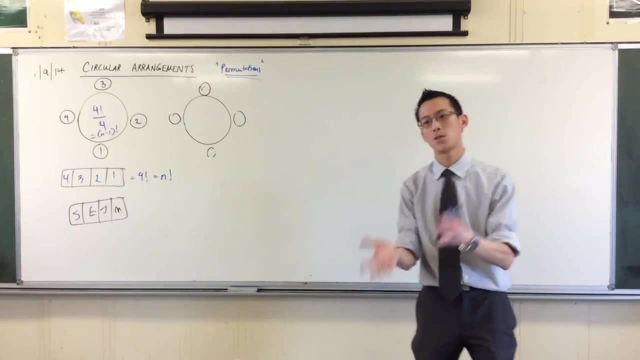 the way I like to think about it, because it fits into how we think about conditions and all that kind of thing is. you think about the circle as a condition And you know when we look at arrangements or probability, you always deal with conditions first. They change. 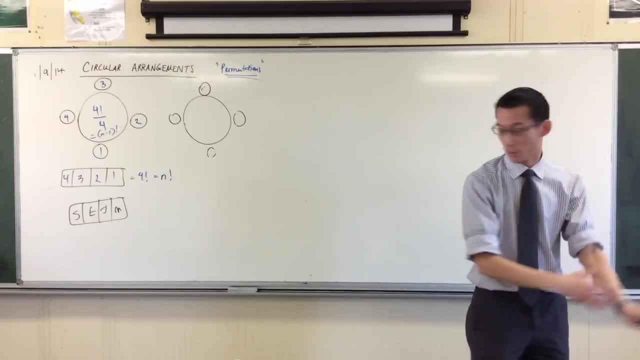 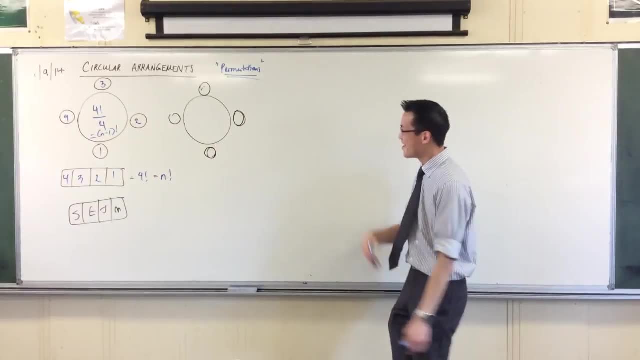 your sample space or whatever, and then you let the situation unfold. So here's the way I would pick it. okay, When you think about that first person- I think it was Savinda. okay, When you think about that first person. really, all of these changes are going to be. 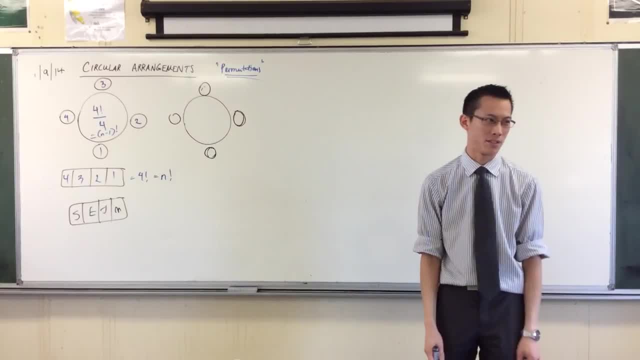 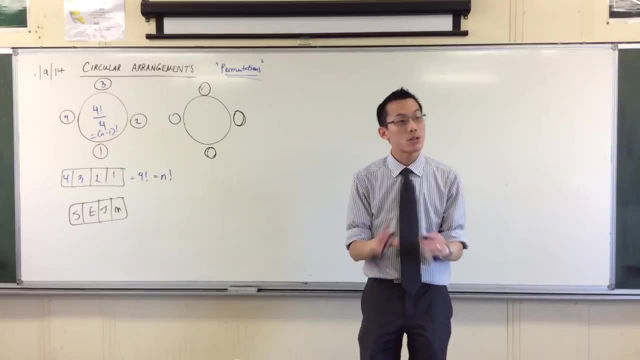 identical. The chairs are identical. They don't actually have any differences between them, okay, Because if we sit him here, we just rotate the table and he's at another chair. Well, it's the same thing, okay. So here's the approach I have You take your. 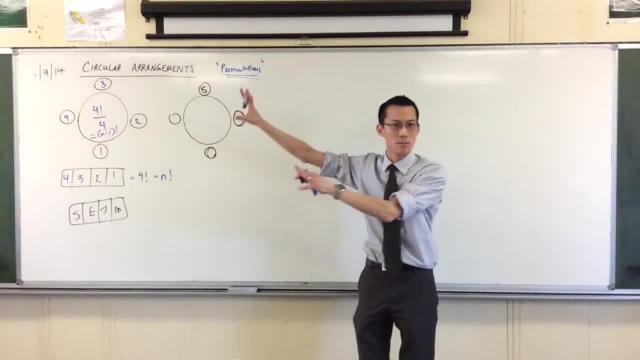 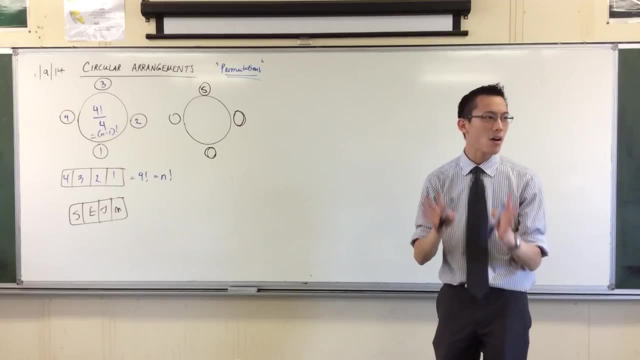 first person and you just lock them in place. You lock them in place, okay Now. you don't worry about where they're going to sit, because all of the places are the same to them. okay, Now, what are you going to do? Well, you have three things to fill and you have three objects. 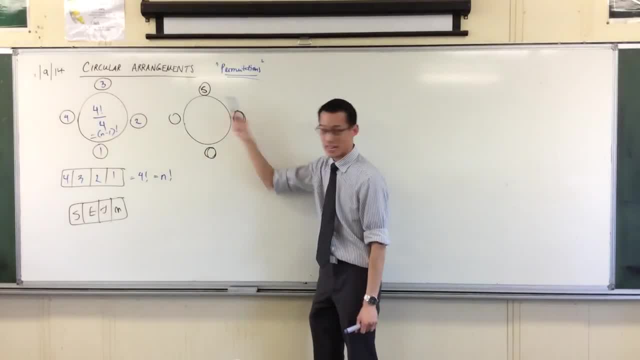 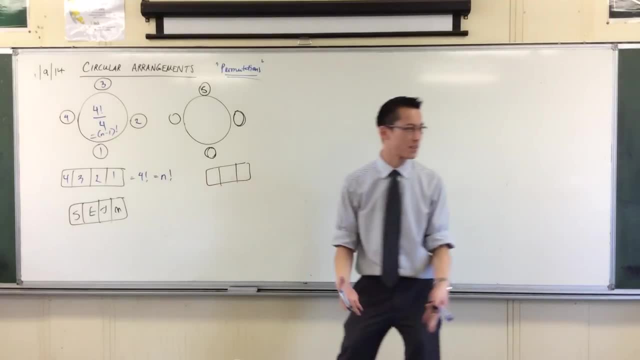 to fill them with And, unlike this situation, you can do this, You can do this, You can rotate these right. This is a line like this, right? It's just that, well, there's only three spots. There's your n minus 1, okay, So your first person, you just lock. 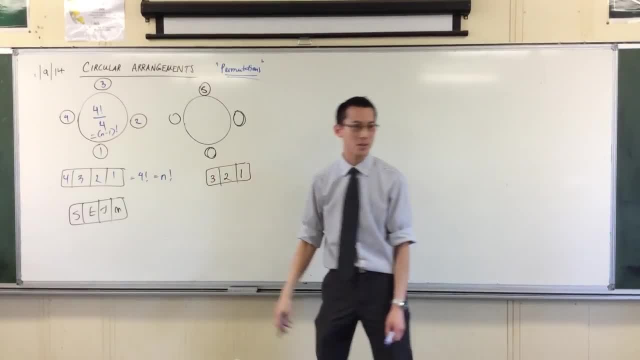 him in. and then there are three: two, one ways to arrange what's left, Three, factorial. Does that make sense?